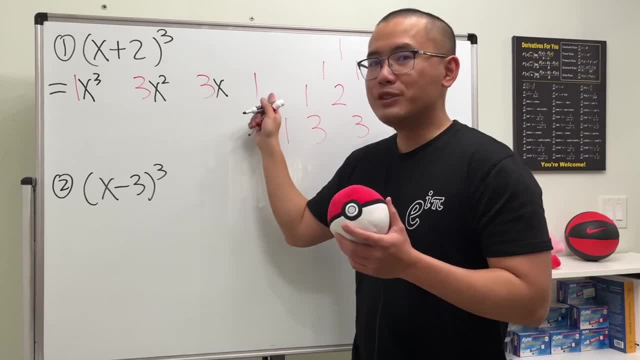 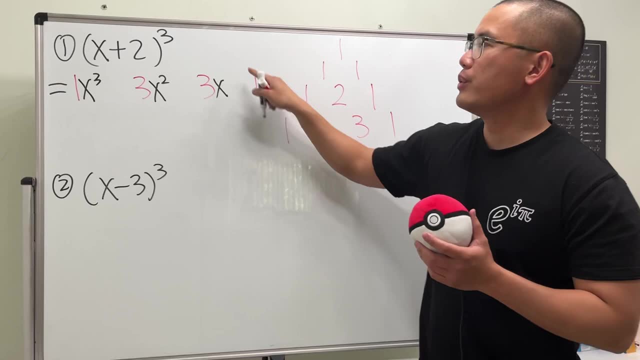 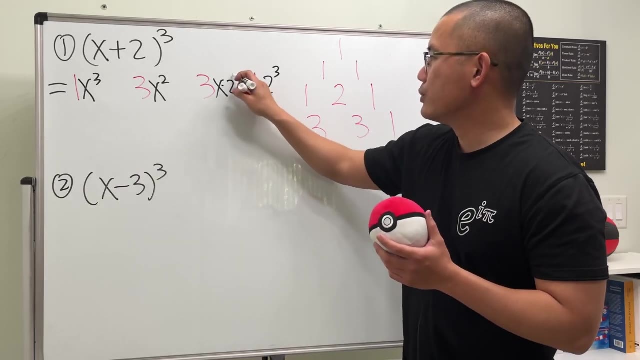 no, x, all right, And then, once we are here, the second term is 2,. yeah, So I'm going to start with 2, right here, and multiplying 2 to the third power, and then we go back and each time the power goes down by 1.. So, multiply by 2 to the second, multiply by 2,. 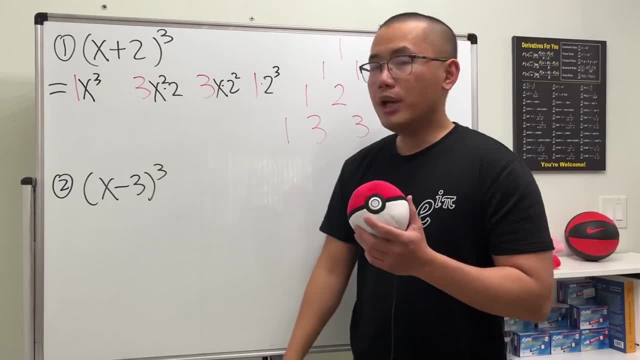 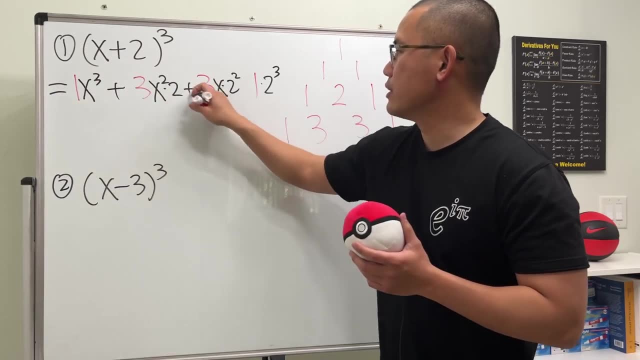 and then multiply by no 2s And we are almost done. Pay attention to the sign here. This is just a sum, right? So we're just going to add them up. So we just have addition, addition, addition And finally we'll just multiply things out. Here we have just x to the third power. 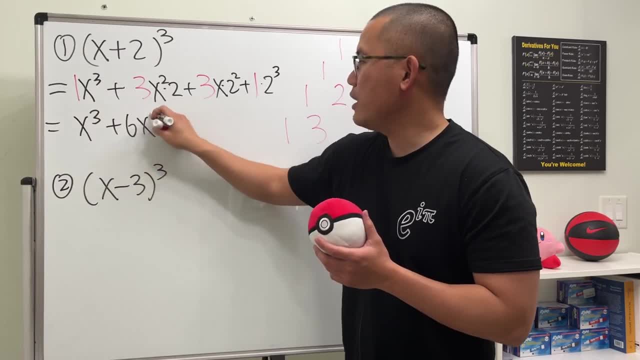 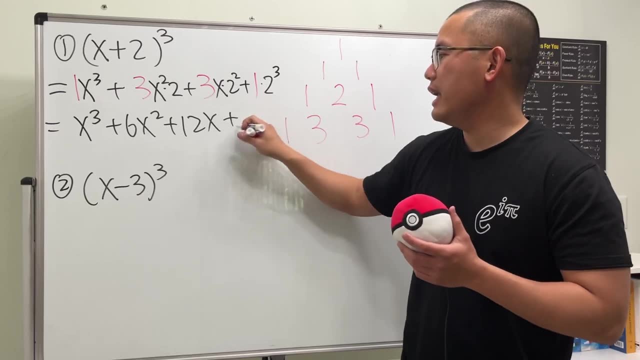 and then this is 2 times 3, so we have 6x squared, and this is 4 times 3, which is 12x. and lastly, 2 to the third power is 8 times 1.. Doesn't matter, of course, So this right here. 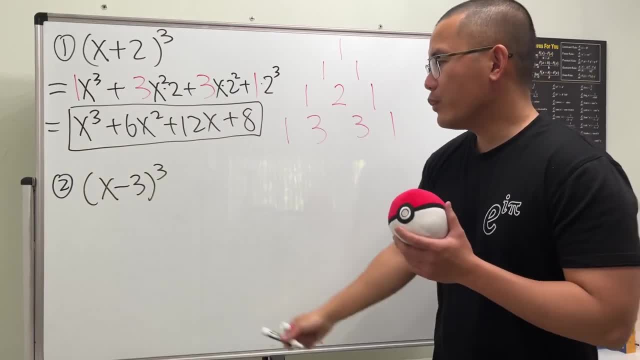 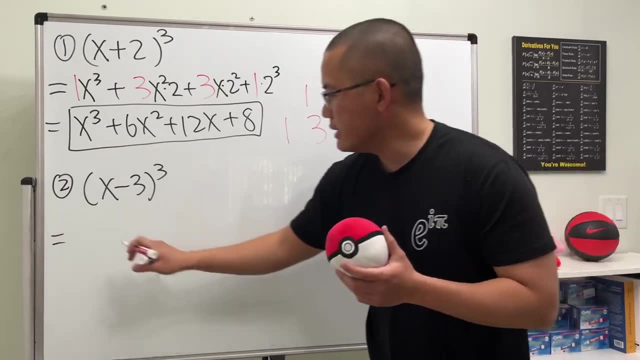 is it Now for the second one? we have x minus 3 to the third power. The steps are the same. Let's go ahead and just make that work. We have 1,, 3,, 3, 1.. Then we start with x to the third power. 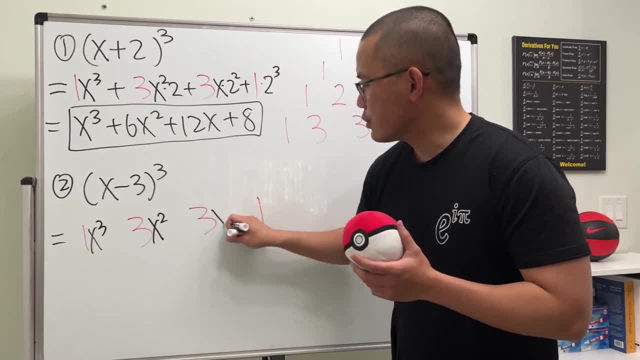 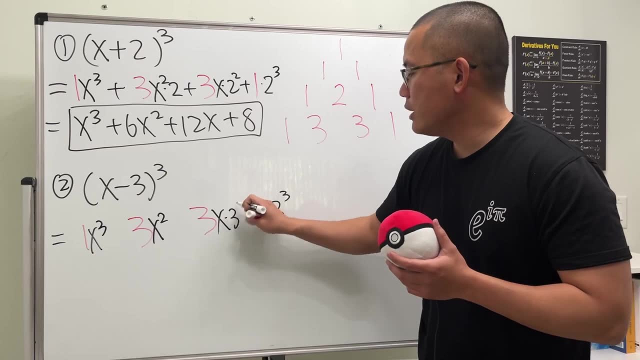 x to the third power, x squared x to the first and no x. And then I'm just going to look at the 3 right here: multiply by 3 to the third power, multiply by 3 to the second power. multiply by 3. 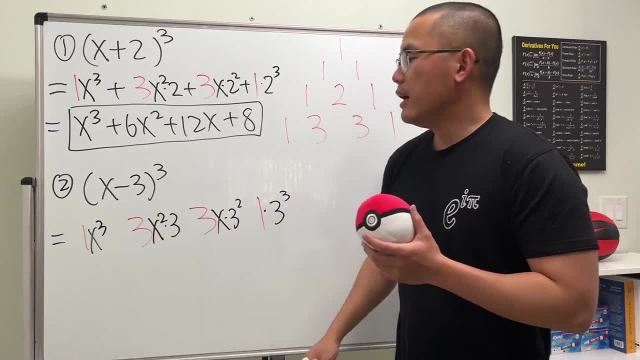 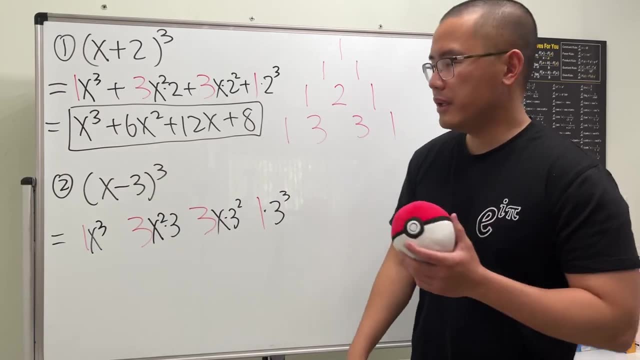 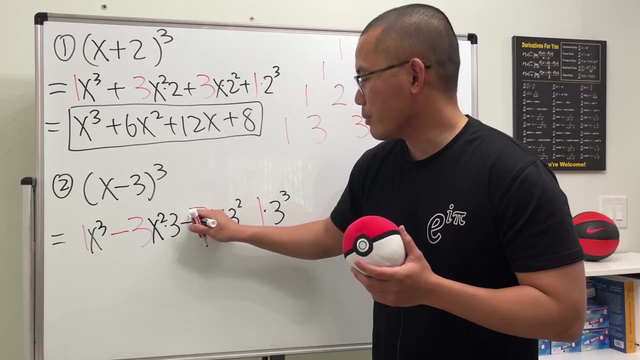 to the first power and multiply no 3.. Now here's the thing. How are we going to put on a sign when we have a subtraction here? The quick way to remember it is the alternates. So you see the right here, The next one will be minus, and then it alternates. 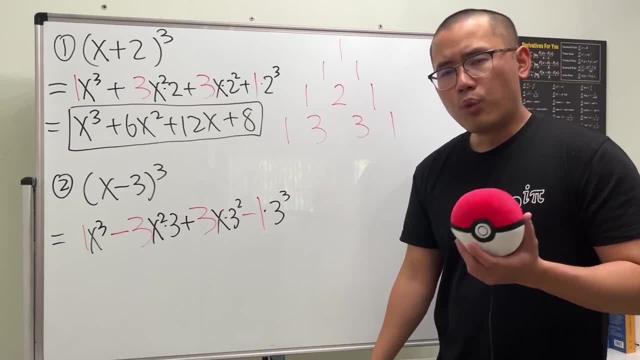 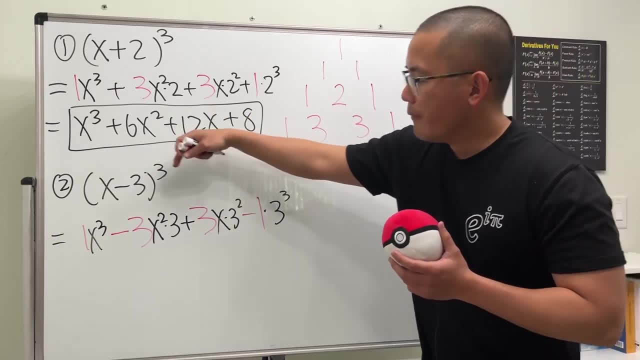 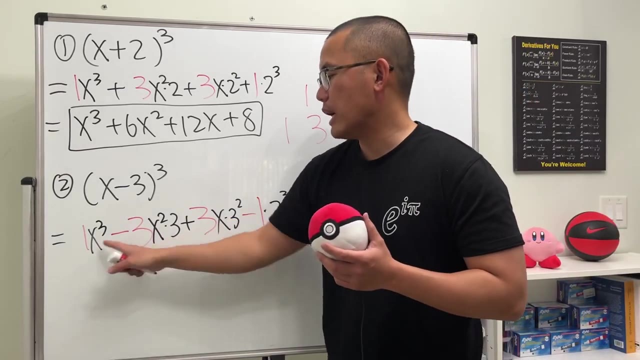 So plus and then minus, just like that. Why, though? Well, if you take negative 3 to the third power, that will give you negative. That's why Negative 3 to the second power is positive. Yeah, same thing, But I think the quick way to do it is just make sure you alternate the signs, like: 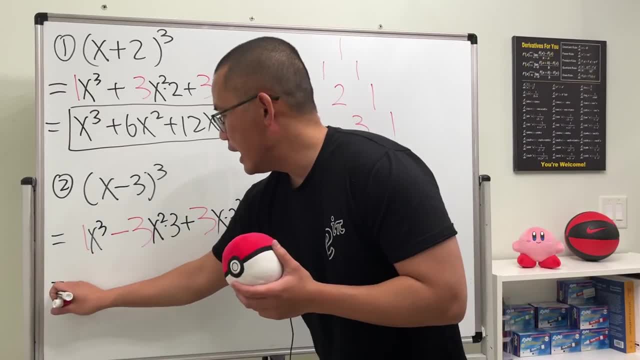 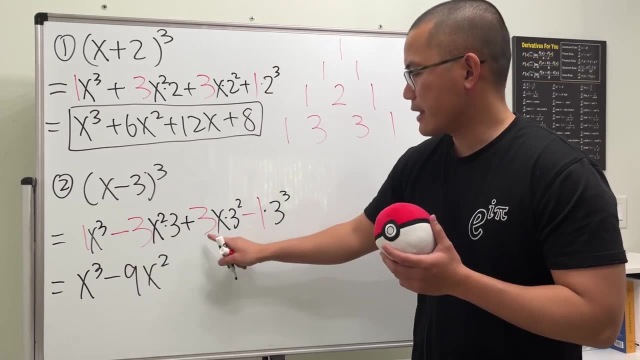 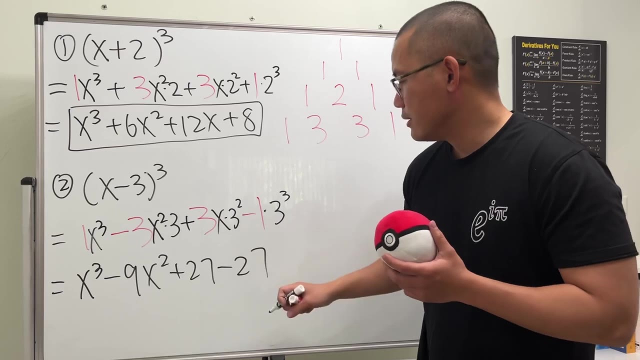 this. And lastly, we just have to multiply the out and we will get x to the third power. This and that is 9, and then we have x. squared, This is 9 times 3.. We have 27.. And then again, 3 to the third power is 27 times 1.. And that's minus. Oh, it's 27x.